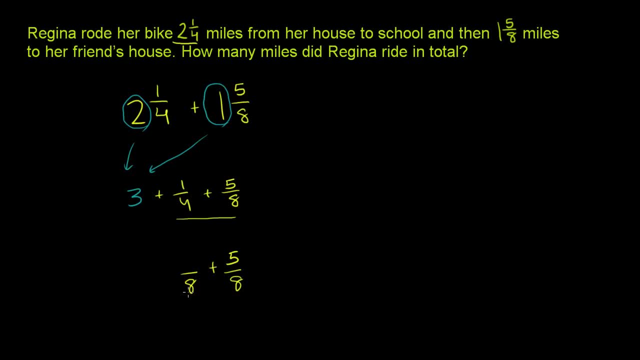 Now, to go from a denominator of 4 to 8, you have to multiply the denominator by 2.. So we also need to multiply the numerator by 2.. So 1 times 2 is 2. And of course we still have this 3 out there. 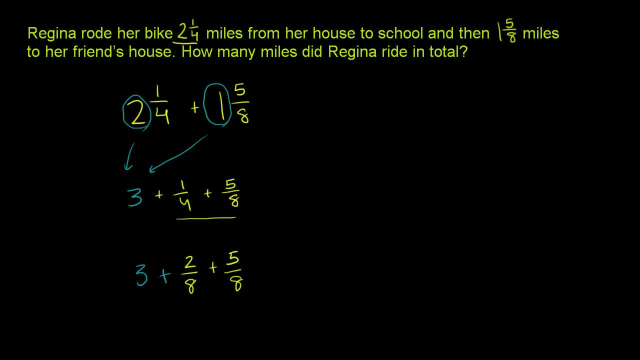 So 2 and 1 fourth plus 1 and 5 eighths is the same thing as this right here, And this is equal to, we have our 3, and then with the plus, and then over 8, we add the 2 plus 5.. 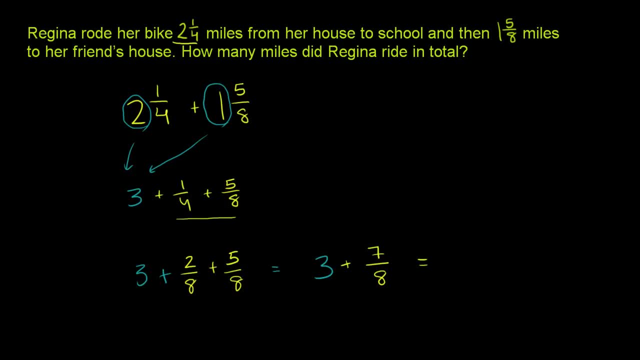 We have 7 eighths, So this is going to be equal to 3 and 7 eighths miles. She wrote a total of 3 and 7 eighths miles. Now I want to make one thing very clear. 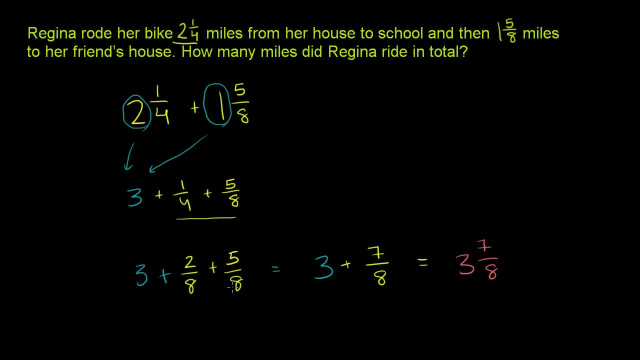 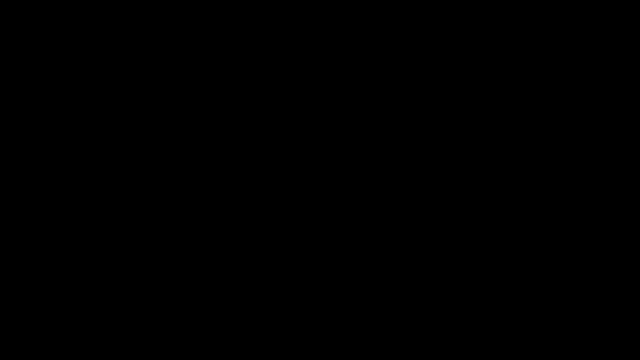 So far, when we've been adding these mixed numbers, the fraction part always ended up as a proper fraction. The numerator was smaller than the denominator. But I want to do a quick example to show you what do you do when the numerator is not. 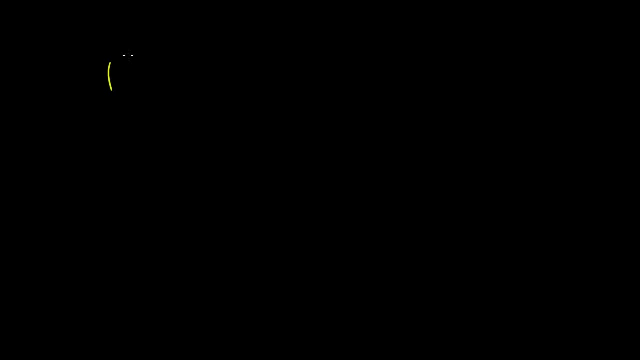 smaller than the denominator. So let's say we had 1 and 5 eighths plus 2 and 4 over 8.. So if you add just the whole number- parts 1 plus 2, you get 3, plus 5 eighths plus 4 eighths. 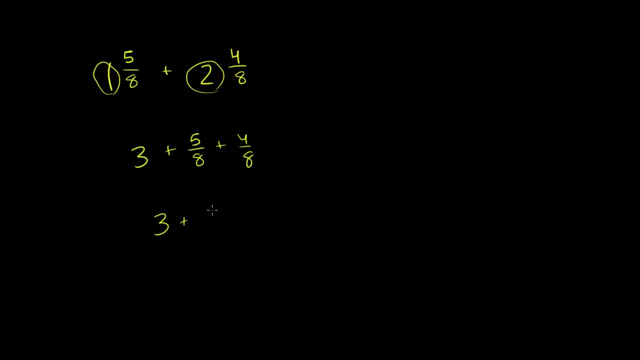 5 eighths plus 4 eighths is 9 eighths, So you get 3 plus 9 eighths. Now it would be really strange to just say: OK, that's the same thing as 3 and 9 eighths. 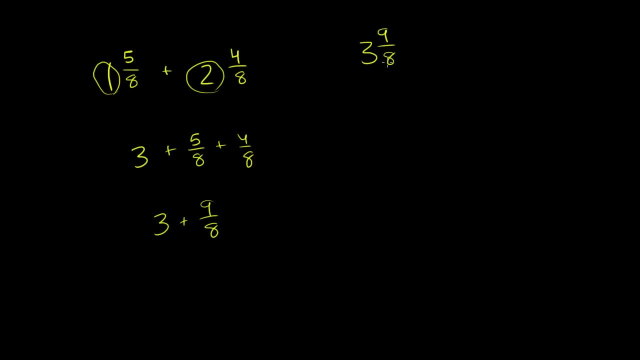 Because you have a mixed number with a whole number and an improper fraction. If you're going through the trouble of making it a mixed number, the fraction better be a proper fraction. So what you need to do is rewrite 9- eighths. 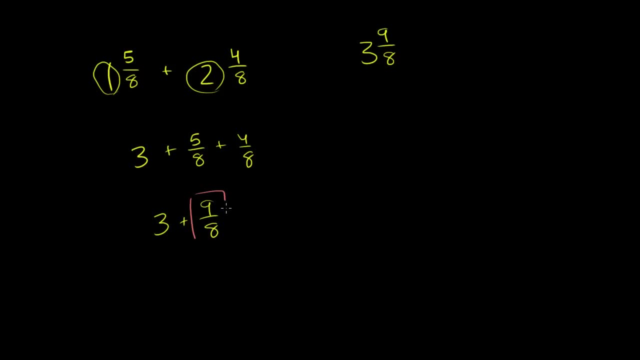 And we know that 9 eighths is the same thing as 1 and 1 eighth. right 8 goes into 9, one time with 1 left over, So it's 1 and 1 eighth. So this is the same thing as 3 plus 1 and 1 eighths. 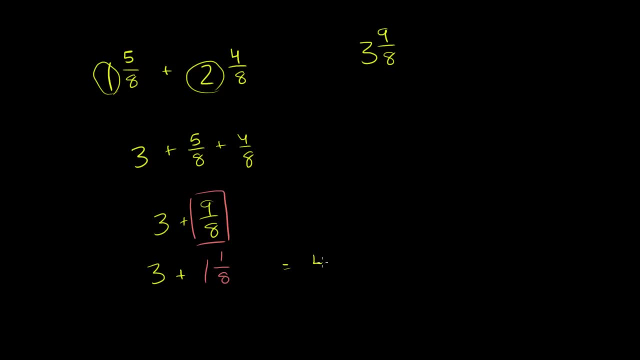 So now we can add the whole number parts. 3 plus 1 is equal to 4.. And then you have your 1 eighth over there: 4 and 1 eighth. I just want to give you that special circumstance when your fraction part ends up improper.